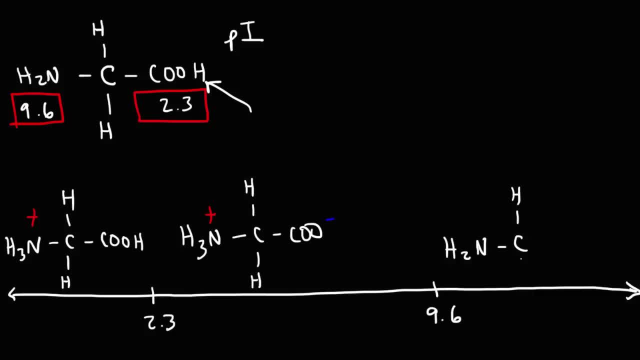 deprotonated And this will now be the dominant form of the amino acid. So on the left the net charge is plus 1.. In the middle it's 0, and on the right the net charge is minus 1.. 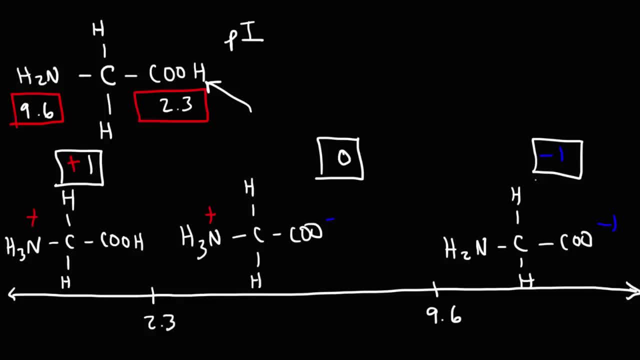 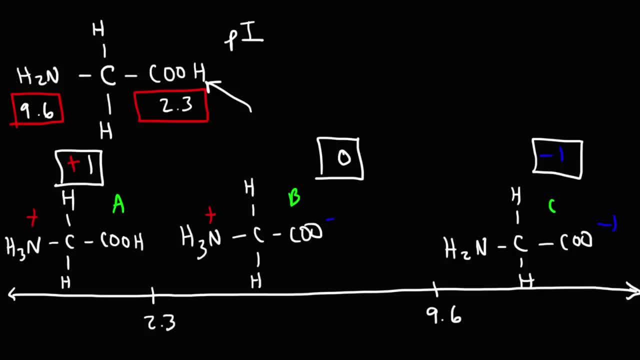 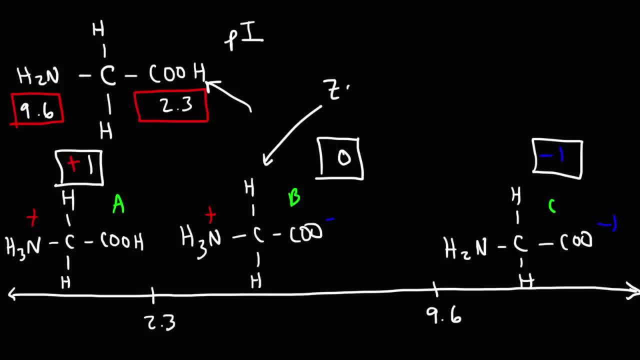 negative charge. So structure B is the zwitter ion. Now, in order to calculate the PI, we need to take the average of the pKa values to the left and to the right of the zwitter ion. So, to the left of the zwitter ion, the pKa value, or pKa1. 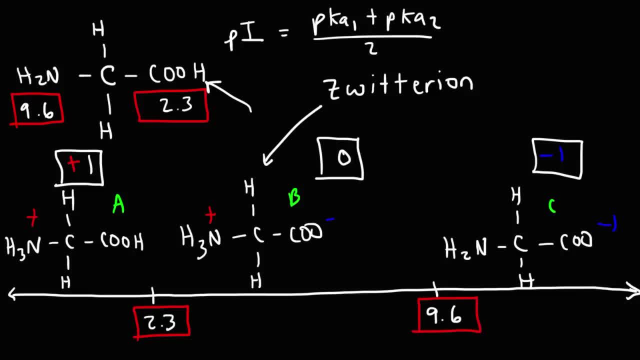 is 2.3 and to the right of it it's 9.6.. So it's going to be 2.3 plus 9.6 divided by 2.. So that's going to be: 2 plus 9 is 11! 0.6 plus .3.. that's 9.提到9.. 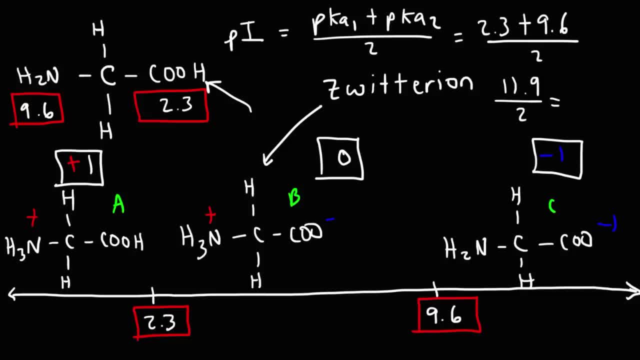 so it's 11.9 Lcm point nine divided by two. 11.9 divided by two is about five point nine five. so that would be the isoelectric point of this particular amino acid. so at a pH of five point nine five, the dominant form of the amino acid will be almost. 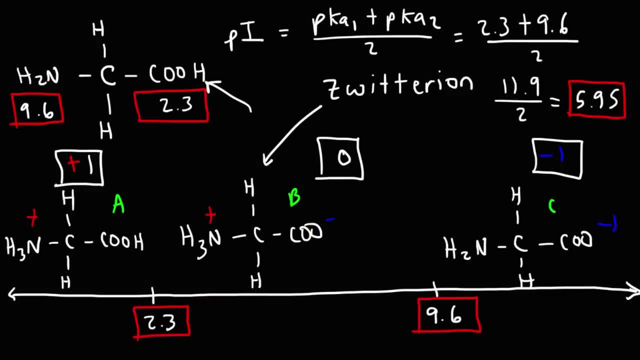 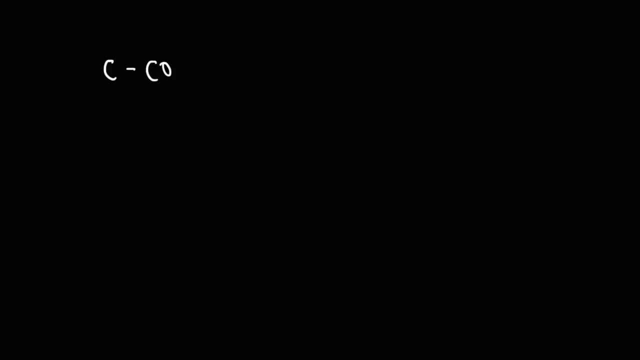 completely the zwitter ion. now let's work on another example for the sake of practice. so here is another amino acid. like all amino acids, it has a carbic acid functional group, an amino group, a hydrogen atom, and the R group is going to look like this: 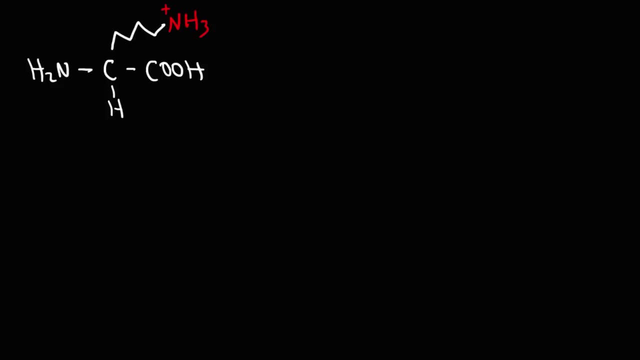 so what type of amino acid do we have? would you say? this is a polar amino acid, nonpolar acidic, basic aromatic. this is lysine and because we have an amino group as the R group, it's going to be a basic amino acid. now, the pka values for lysine are 2.18 for the carbic acid. 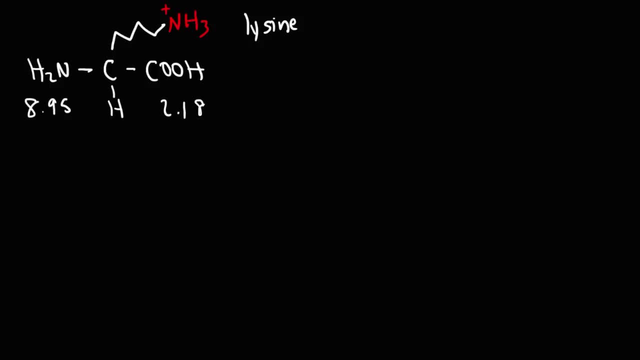 functional group, eight point nine five for the amino group and ten point five for the amine on the side chain on the R group. so, using these three values, go ahead and calculate the isoelectric point of this water ion for this amino acid. feel free to pause the video and work on it. so let's create a number line and let's put 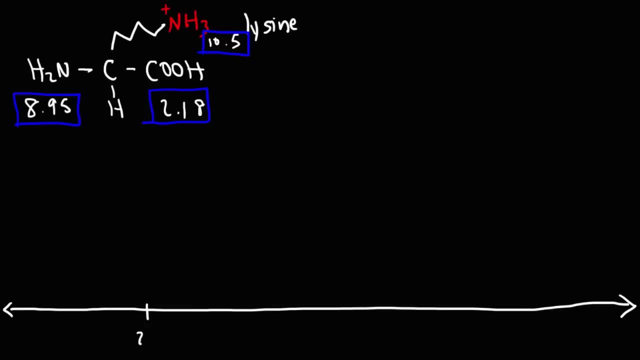 the pKa values. So here this is going to be 2.18.. The second pKa value is 8.95 and the third one 10.5.. Now let's draw each of the four forms of lysine, So when the pH is less than 2.18,. 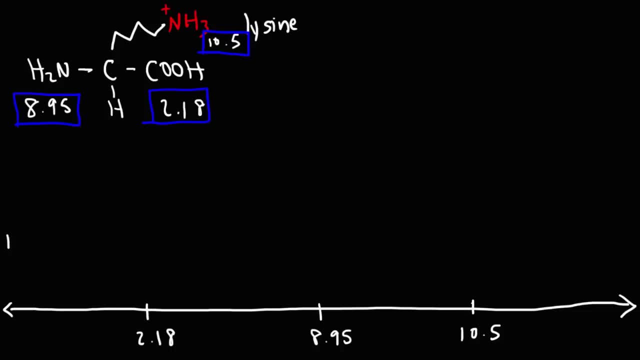 this amino acid will be fully protonated. Each nitrogen atom will have a positive charge, So this will be the dominant form of lysine at a pH below 2.18.. Now, at a pH between 2.18 and 8.95,. 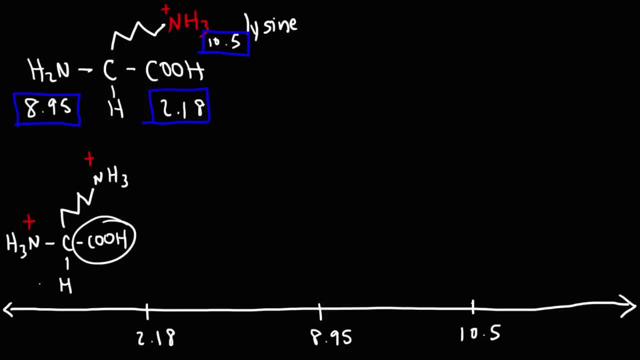 since we're going past the pKa values, we're going to draw each of the four forms of lysine So at a pH below 2.18,. since we're going past this pKa, the carboxylic acid is going to lose. 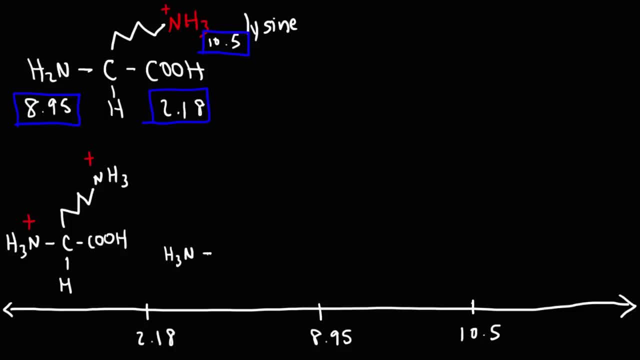 the hydrogen, And so the structure that we're going to get is going to look like this: Each nitrogen atom will still have a positive charge, but now the carboxylic acid functional group is deprotonated, So it carries a negative charge. We have a carboxylate group now. 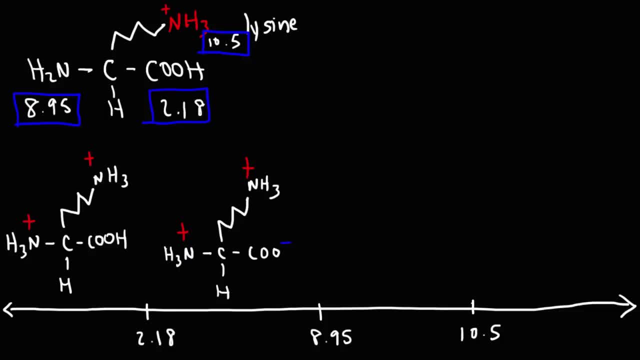 Now, once we go past a pH of 8.95,, the nitrogen group here will lose a proton, So instead of being H3N, it's going to be H2N, And so we have this structure And then finally, at a pH beyond 10.5,. 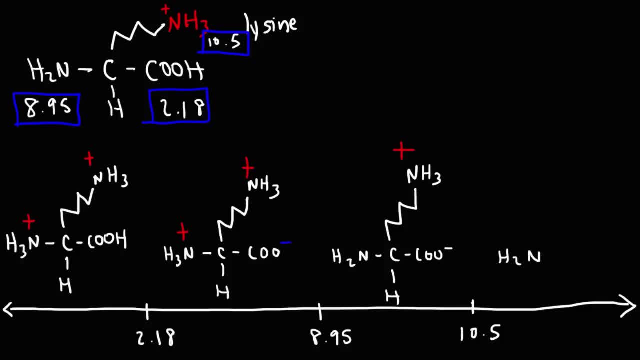 we're going to have a carboxylate group. The last nitrogen at the top will lose its proton. So now we can determine the net charge of the amino acids. So on the left we can see that the charge is positive 2,. 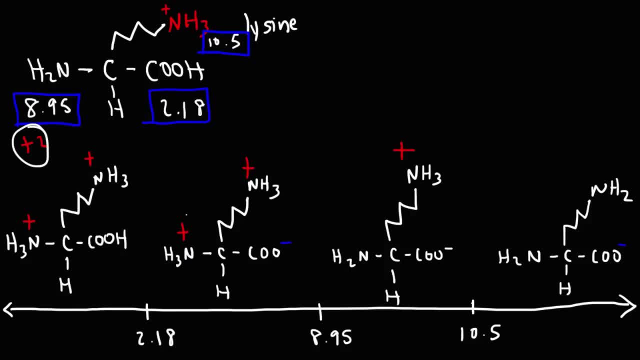 because there's a plus and a plus. The next one it's plus 2, minus 1, so that's positive 1.. And it's always going to decrease by one from here on. So this is plus one and minus one, that's zero. 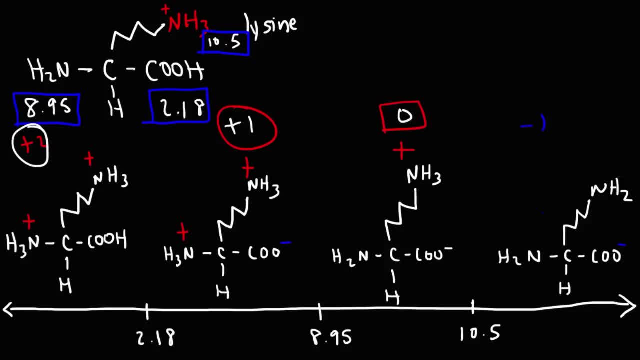 And for the last one we can see that it's negative one. So this right here is a zwitter ion, Because the total charge is zero. we have a positive charge and the negative charge. So to calculate the isoelectric point of the zwitter ion we need to average these two pKa values. 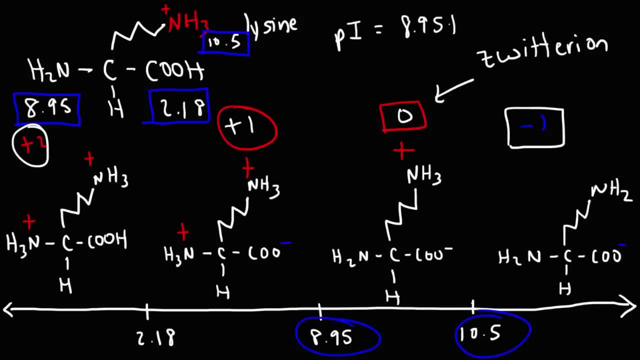 So it's going to be 8.95 plus 10.5 divided by two. So 8.95 plus 10.5, that's 19.45 divided by two. This gives us an isoelectric point of nine. 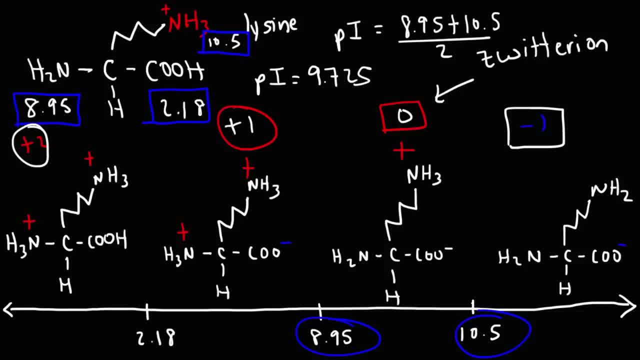 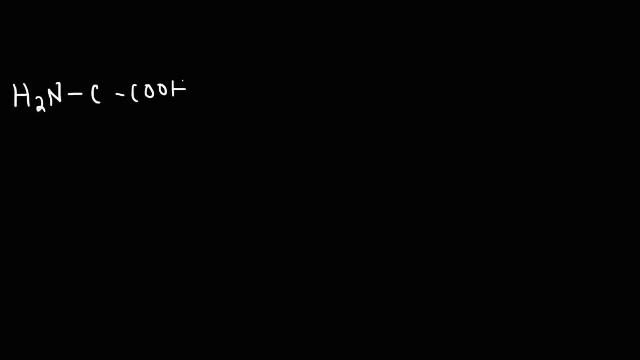 So that's how you can determine the isoelectric point of an amino acid. Now, for the sake of practice, let's work on one more example. So the amino acid under consideration is called tyrosine, Tyrosine, Tyrosine. 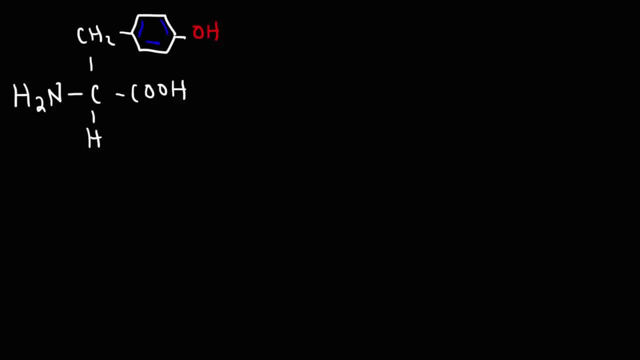 It has an aromatic ring with a hydroxyl group attached to it. The pKa of the carboxylic acid is about 2.2.. For the amino group, it's 9.1.. Now for the hydroxyl group. most phenol groups have a pKa of 10.. 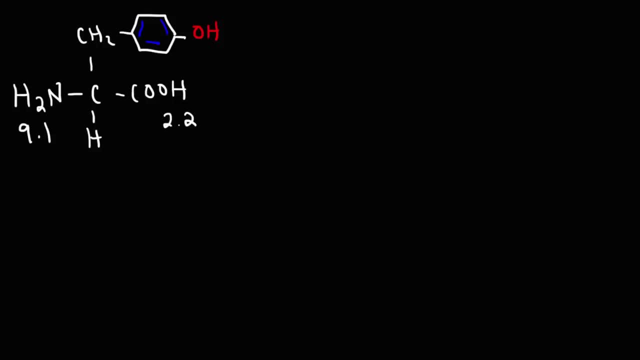 Some textbooks, just you know, says that this is 10.5,, 10.9,, 10.. It's somewhere around 10, but for the sake of simplicity let's say it's 10.5.. So, using this information, calculate the isoelectric point of tyrosine. 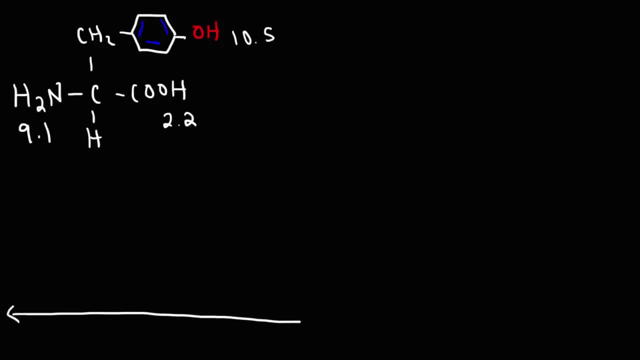 So let's begin with a number line. So we're going to have 2.2,, 9.1, and 10.5.. So there's four structures to draw: 1,, 2,, 3, 4.. 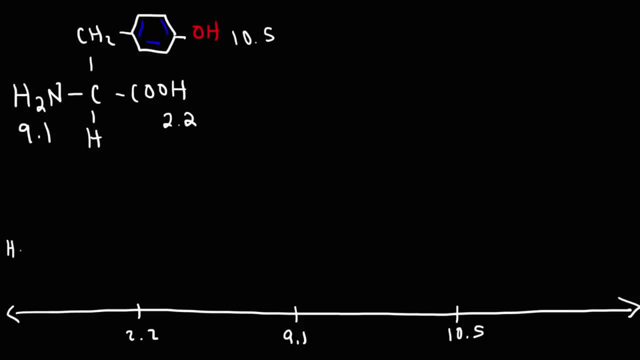 So, starting with the first one, everything is going to be protonated: The amino group will have a positive, The carboxylic acid will have a positive charge, The carboxylic acid will have its hydrogen, And the same is true for the phenol group. 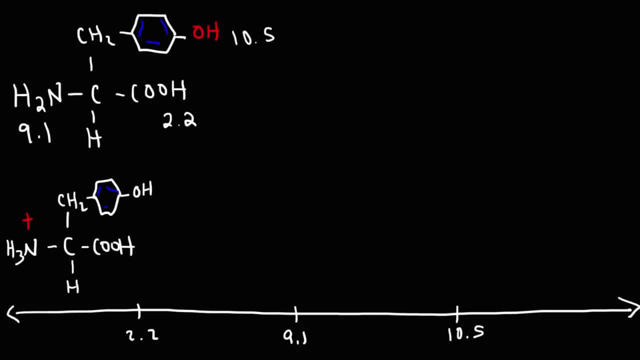 So that's going to be the structure at a pH below 2.2.. Now, once we go past 2.2, the carboxylic acid is going to lose a proton. Hence we're going to lose a proton. 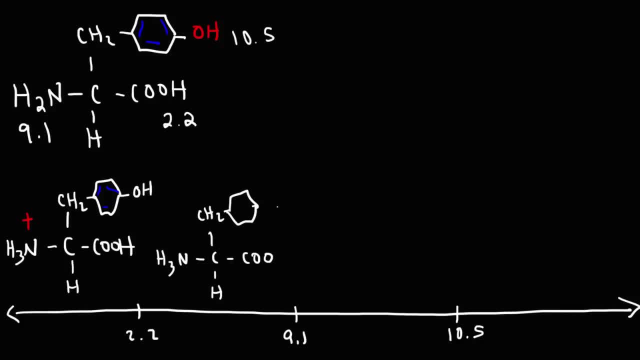 So we're going to get this structure, and so we're going to get this structure. So here we have a negative charge, and here we have a positive charge. Now, past 9.1,, the amino group is going to lose a proton, So it's going to be H2n instead of H3n+.